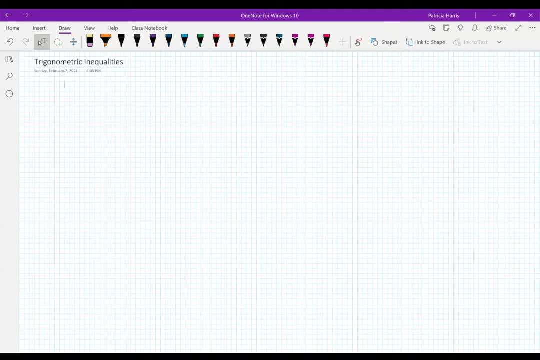 Okay, guys, let's talk quadratic inequalities, trigonometric inequalities. Okay, so usually what I do is I recommend solving these using Desmos because it's nice to get that visual, But for some of you you don't like Desmos. And if it's simple, then you can do it by hand. 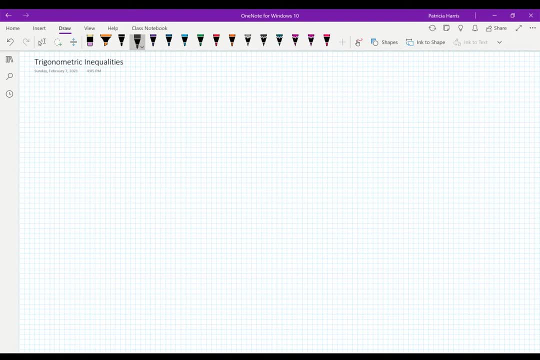 So let's do a couple of simple ones. So we want to find out where sine of x is less than or equal to- okay, one half, Okay. so when you solve any inequality, it has what we call a related equation. Okay, Oops, I'm sorry, I should have said from zero to two pi. Okay, so what we're going to do is we're going to change this to the equation sine x is equal to one half. Okay, so we're going to solve that. So, using the inverse function or the unit circle, we know that sine is one half. 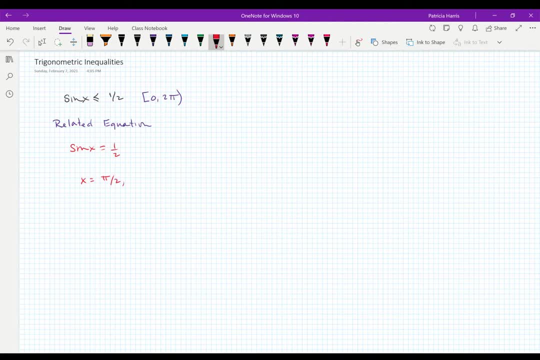 And x is equal to pi over two And it is one half again five pi over six. Actually. no wait, that's not a two, That's a six. Okay, I'm sorry. So pi over six and five pi over six. Okay, so that tells us where it's equal to it. I want to know where it's less than. 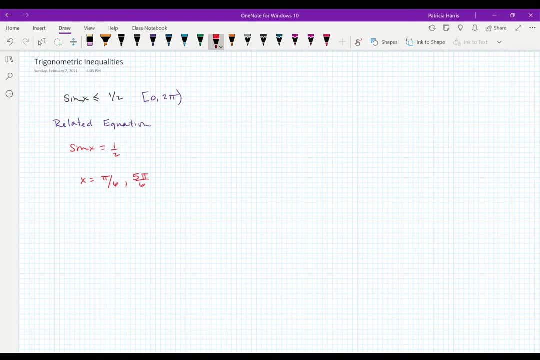 Okay. so if you have a true sense of the unit circle, you know that one sine of x is equal to one half sine oscillates. so when it starts at zero it moves up to one half, crosses the one half mark and then goes all the way up to one, then back down, hits the one half again and 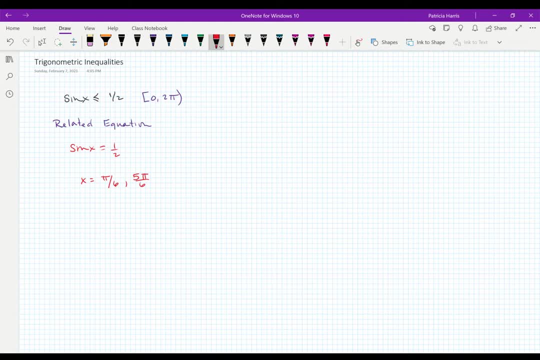 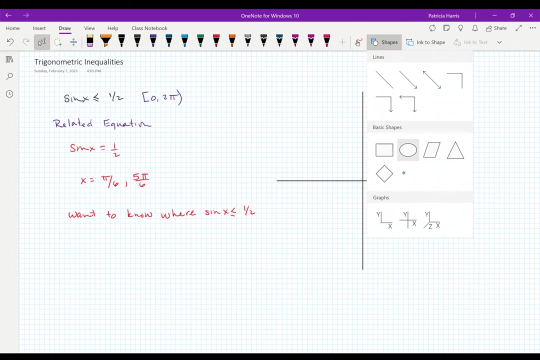 then it goes into the negative. Okay, so we want to know where sine of x is less than or equal to one half. Okay, so, thinking about my unit circle, Oops, Let's see if I can do this, There we go. That works. Okay, so this is zero. this is pi over. two pi, three pi over. 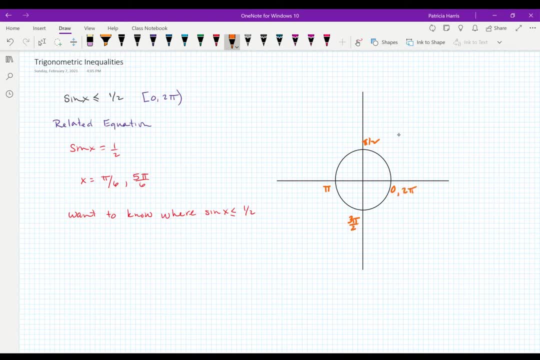 two, and if we go all back around, okay, two, pi. So this right here is pi over six, this right here is five, pi over six. Okay, So if I think about sine starts at sine, at zero equals zero, and then it goes up until: 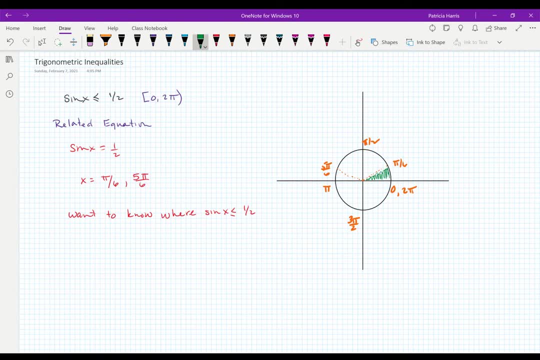 it hits pi over six. Now, at this point it is less than one half. It's below that one half mark. As soon as it hits pi over six, it's above that half mark, Until it comes all the way around to five pi over six. Once it hits five pi over six. 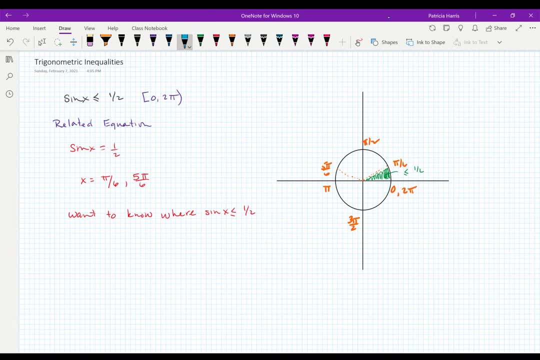 then we get below that one half mark. Okay. so remember, sine at pi is zero. Once it hits the zero it goes down below into the negatives. So that's all less than or equal to one half. Okay, So I can write my answer as zero, because we're solving from zero to pi over six. close. 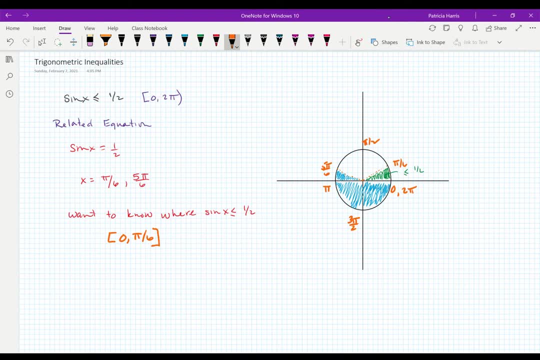 bracket because it's equal to, and then five pi over six to two pi open bracket because of where I'm supposed to find my solution. Okay, Now you could have done this by graphing it on Desmos. So let's try. let's do another simple one and see what happens. Oops, Okay. 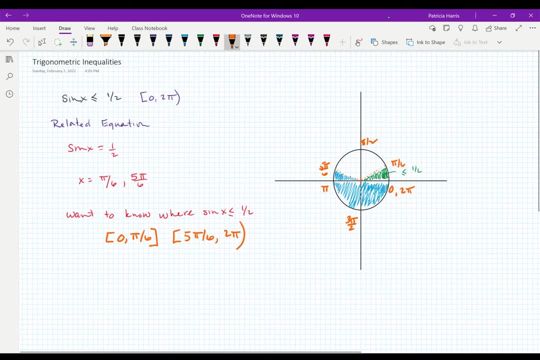 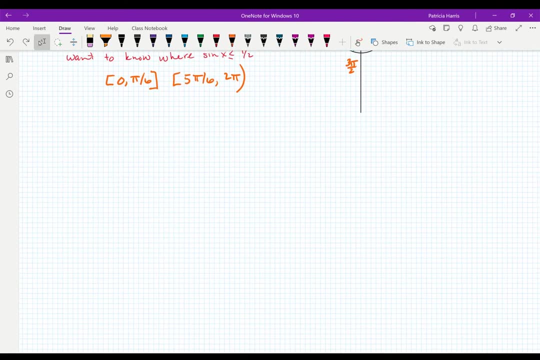 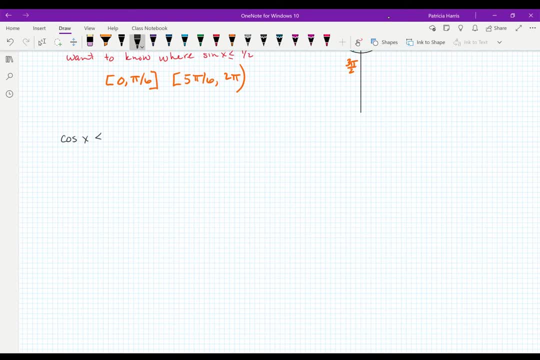 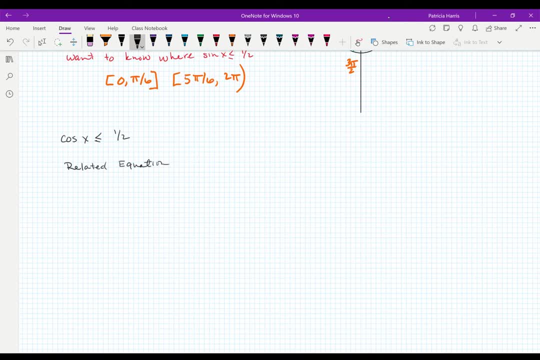 Okay, so cosine is equal to a positive 1 half at pi over 3, and 5 pi over 3.. Okay again, we're going to try to use our unit circle to help out Now what I'm going to do this time. I'm not going to draw my unit circle. 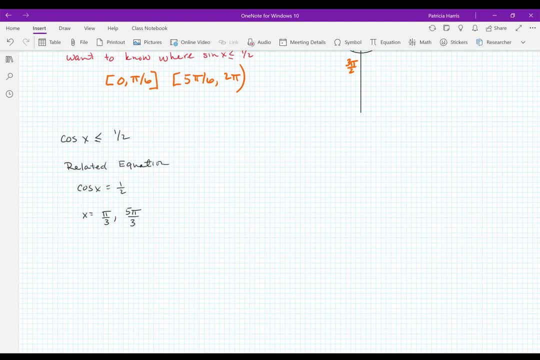 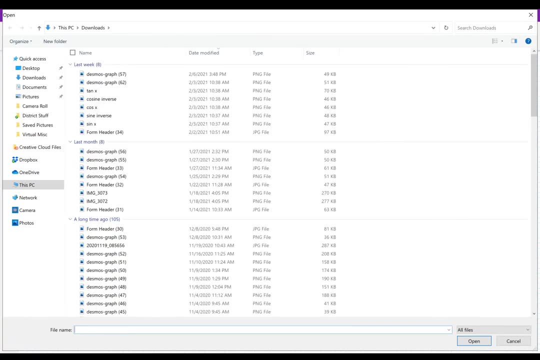 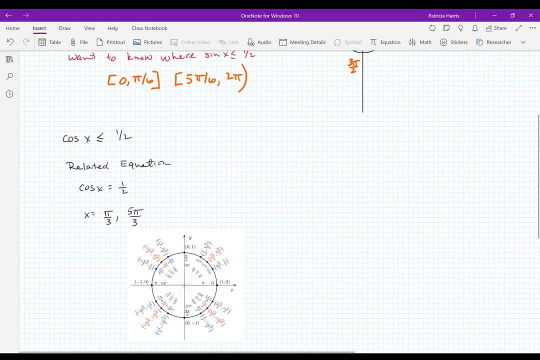 I'm going to use a unit circle that's already been drawn for me So you can see kind of how that would work out. Let's see here. There it is Okay. so a lot of you already have a unit circle, Okay, alright, so we're looking at cosine. 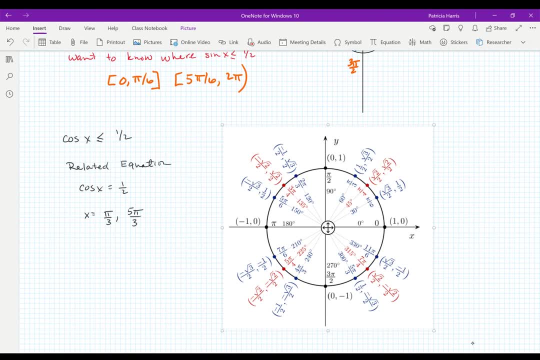 Alright, we have 1 halves at pi over 3, and 5 pi over 3.. Okay, so we want cosine to be less than that. Okay, so less than 1 half would definitely be 0, right Would definitely be negative. 1 half negative, radical 2 over 2..